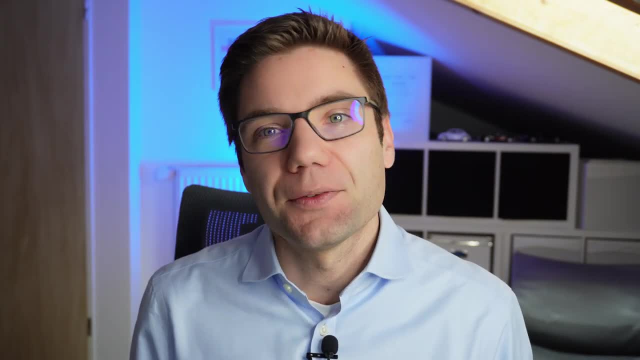 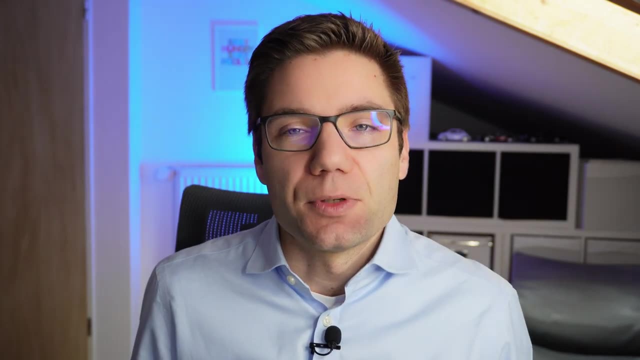 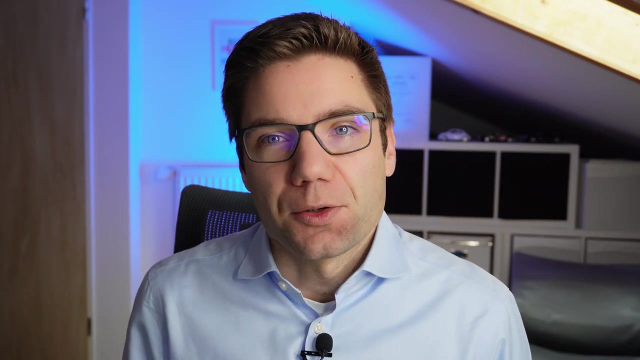 somewhere we all can use home automation, and the nice thing about this is there are a lot of projects already out there. there is a lot of code and project ideas that you can look at, also project solutions that you can start building on and reuse, so that's a great way to start your first embedded. 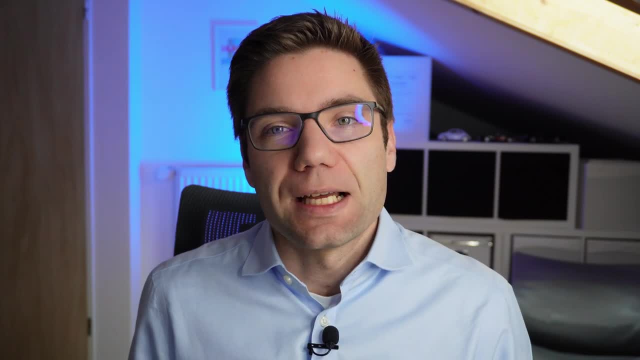 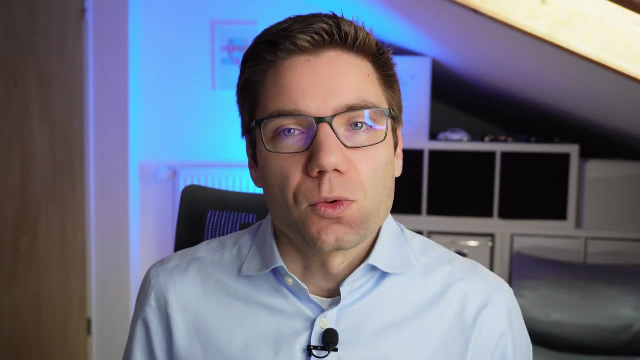 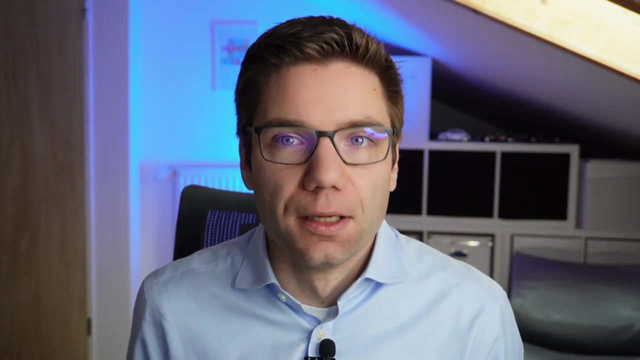 system project And, on the other hand, what's also really nice is there's a lot of controllers out there that you can use and get fairly cheap, like the ESP32 controllers or an Arduino controller or a Raspberry Pi. The second thing that is also a beginner project is a digital clock, A digital 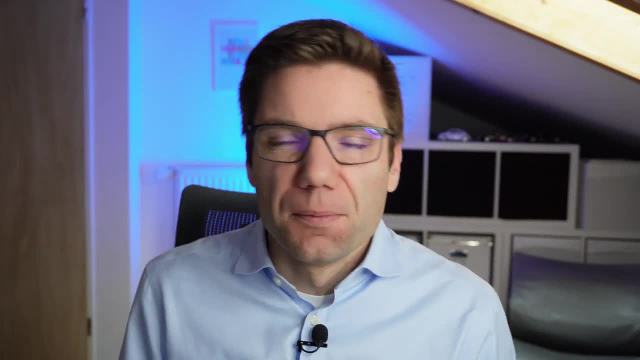 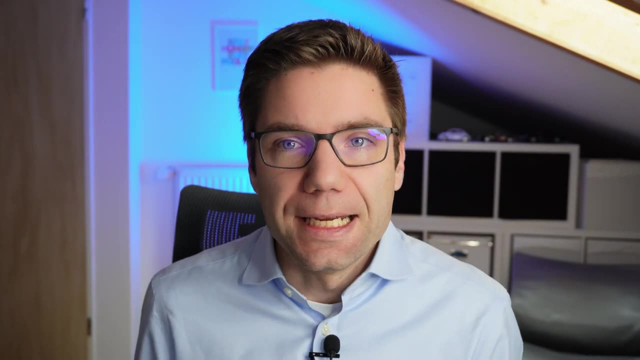 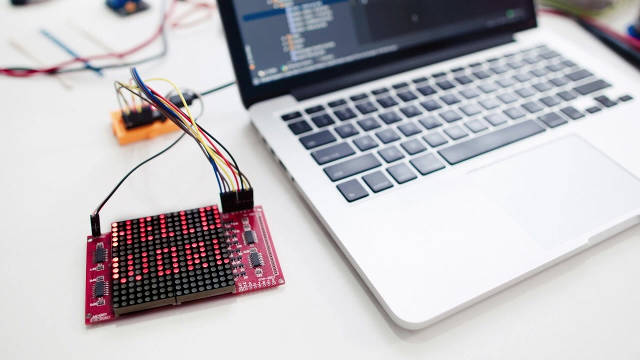 clock, where you can learn about timers, learn about how you actually do real time in a microcontroller and, at the same time, learn how to control a display, Whether that's a seven segment display or whether you want to take it a step further, maybe use an LED matrix display and maybe even extend it by showing your- I don't know- Instagram likes or 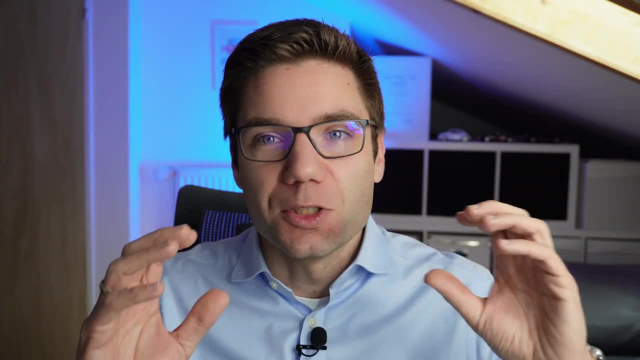 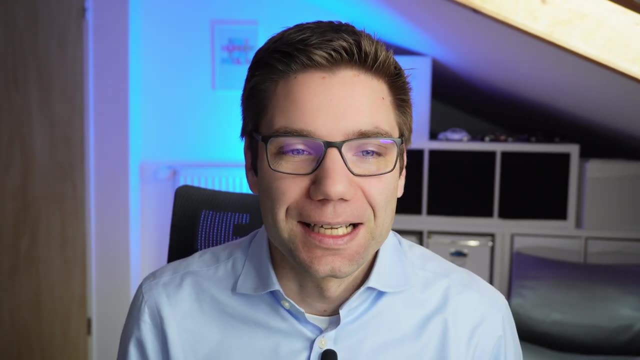 YouTube subscribers. that's a nice project. that's something you can have in your living room and show it off to people that visit you, so that's always nice to have something like this. The third one would be a weather station which is similar to the digital clock, but 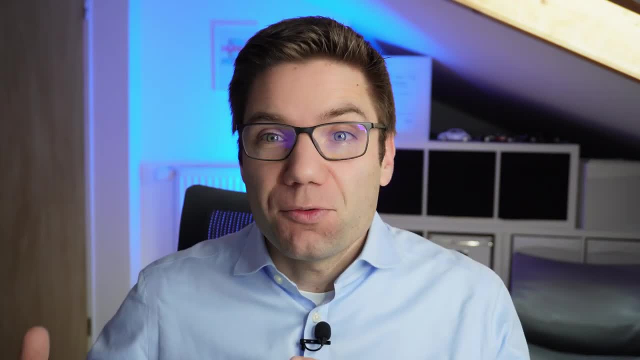 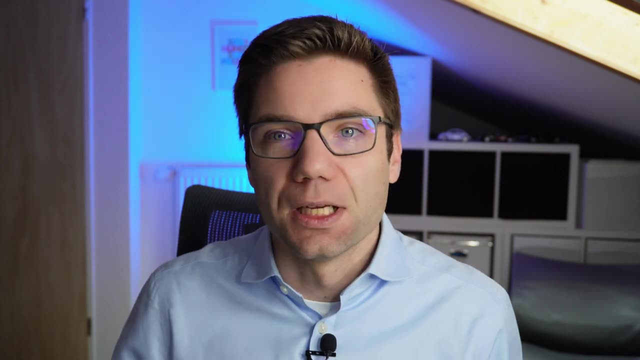 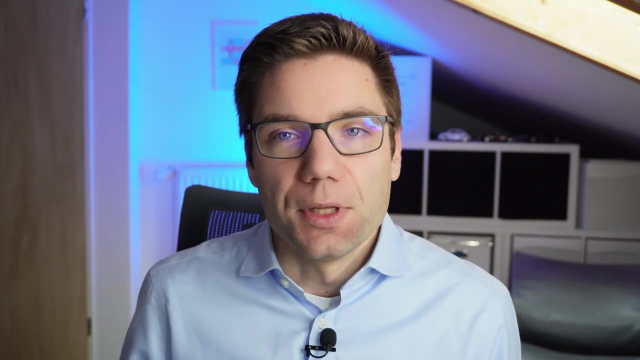 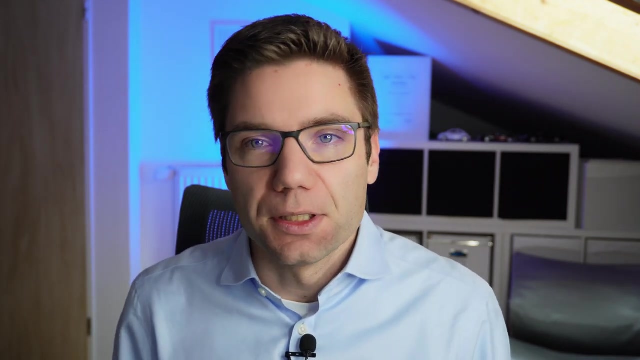 takes it a step further. you have now maybe several sensors that you can use. you have temperature sensors, you have humidity sensors- maybe you are trying to measure air speed, air pressure- and you can also build here your first distributed embedded system where you then actually have multiple microcontrollers, maybe one outdoors, to measure outdoor temperature and outdoor humidity. 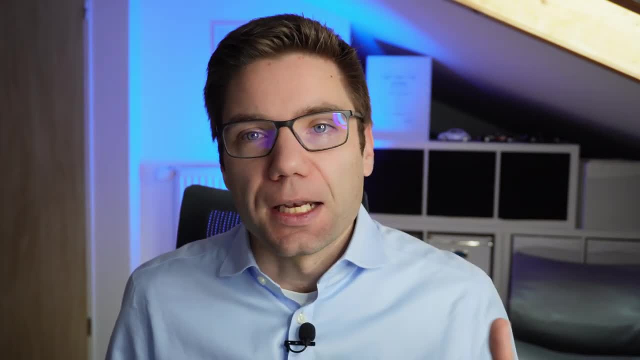 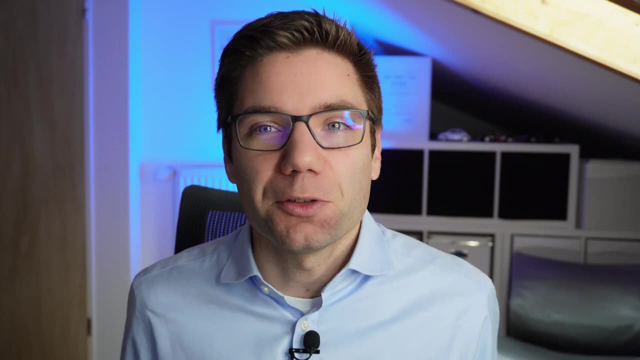 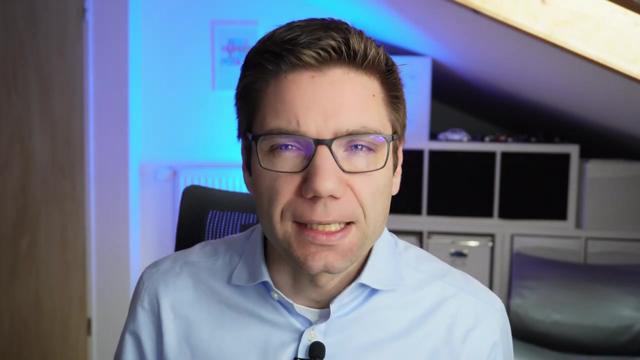 one in your living room, one in your bedroom and you have multiple microcontrollers that then talk to each other via a protocol. also here, you are not the first person that is having this idea. there are a lot of implementations available online that you can look at, get ideas from and then trying to implement it on your own. and fourth, of course, 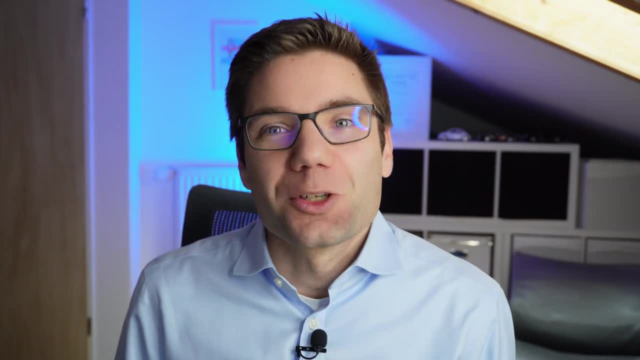 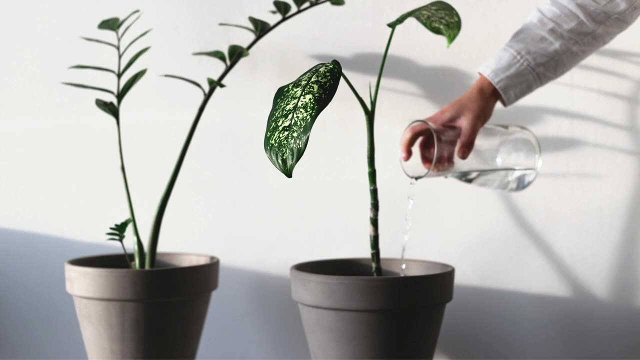 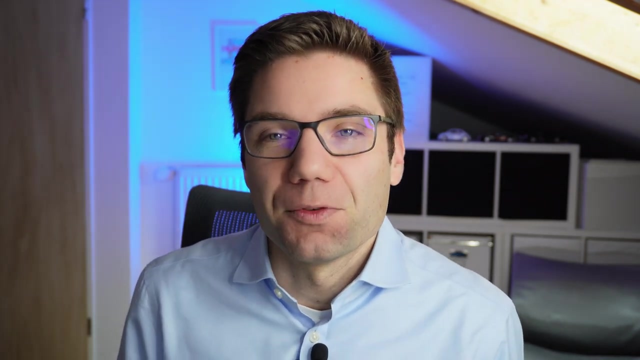 we all like plants and sometimes we all forget to water them- or at least I always forget to water them. and there a great idea is to build an automatic plant watering system, whether that's just measuring the humidity of the soil and it's giving you a reminder whenever your plants need. 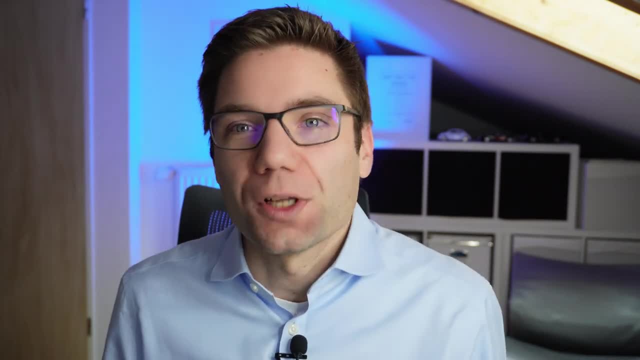 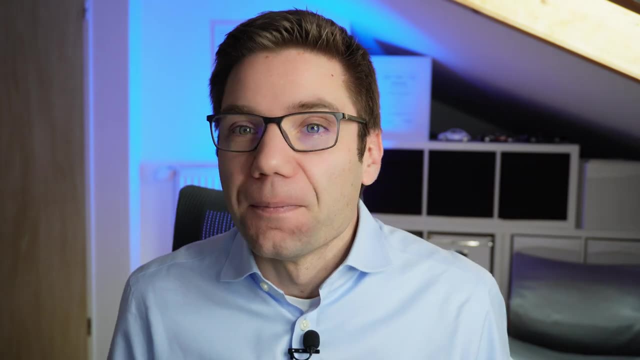 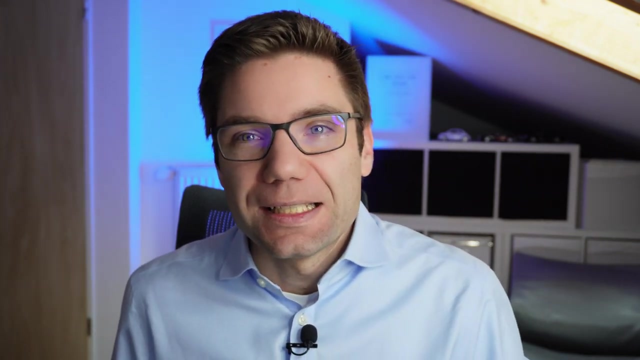 watering, or whether that's even having a small water tank or is already hooked up to your watering system so that you can automatically water your plants. that's up to you. but that's a great system. it's helpful and it saves some plants from dying, If you want to take it up. 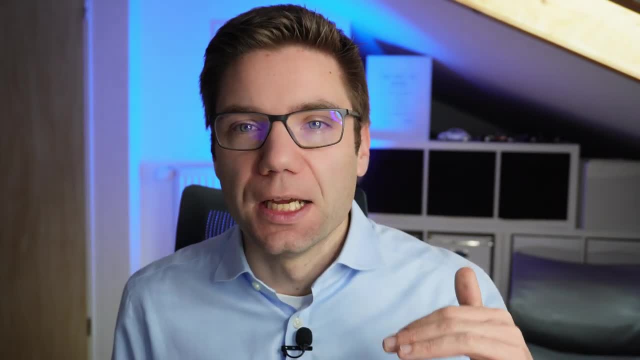 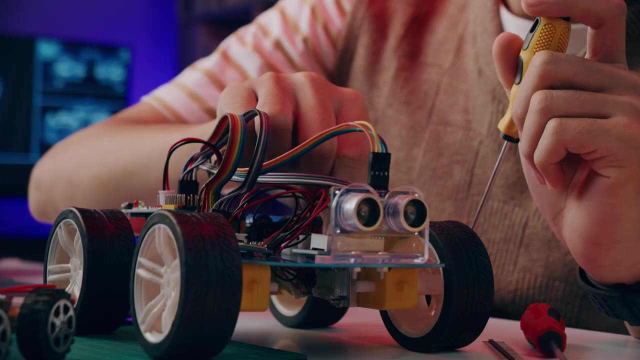 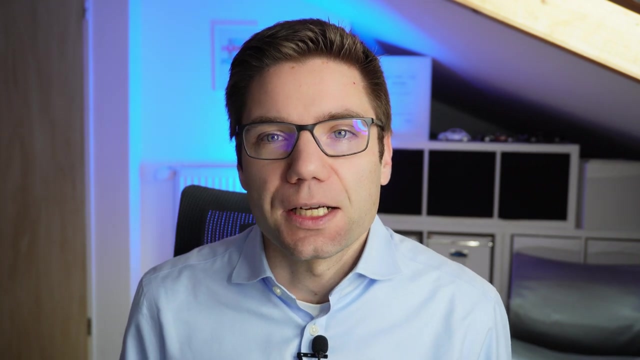 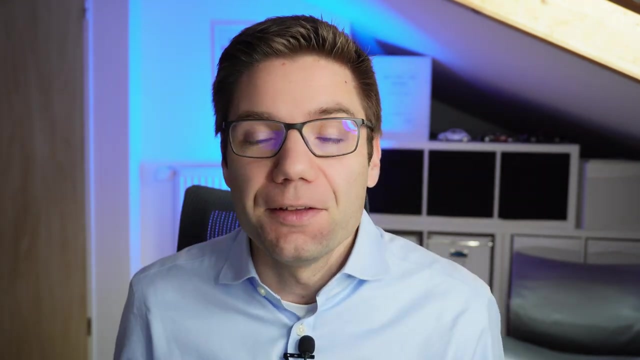 a notch and if you want to have a more advanced project in here it's really going from medium to very advanced. you can start with an autonomous robot. autonomous robots are great. they combine multiple sensors, very nice algorithmic challenges. so they are a great way to really go from this embedded beginner level to a very advanced level and if you have built a fleet, 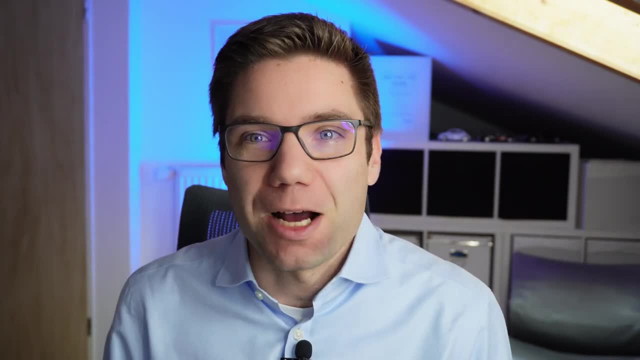 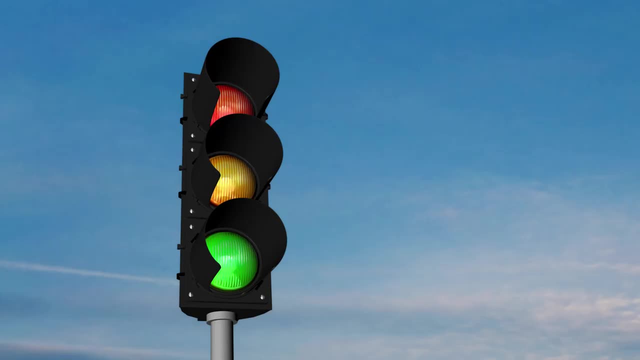 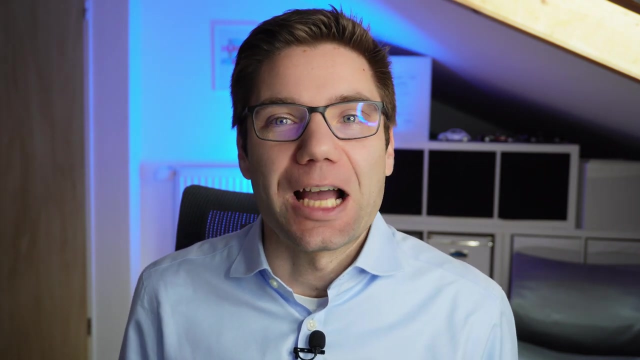 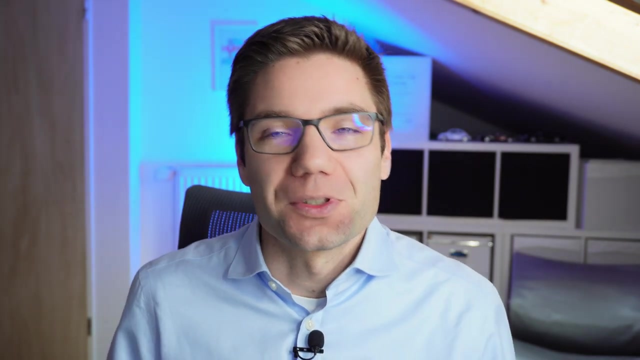 of autonomous cars already that are driving around, then maybe what you could do next is building a autonomous system that then is managing this traffic of autonomous cars, maybe even with a traffic light that is detecting how many cars are already in line. you could have communication between the cars and your traffic management systems. so there's a lot of things that you 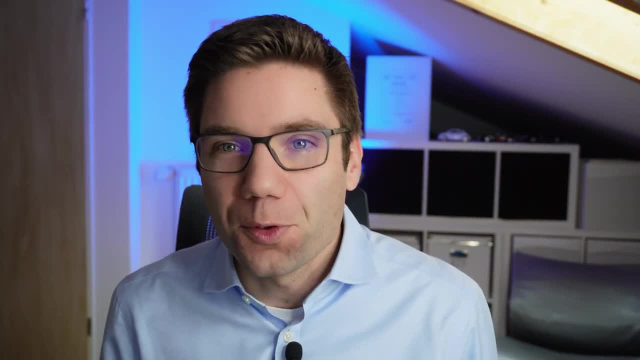 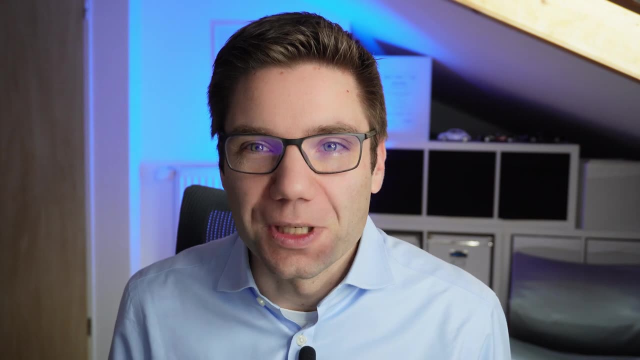 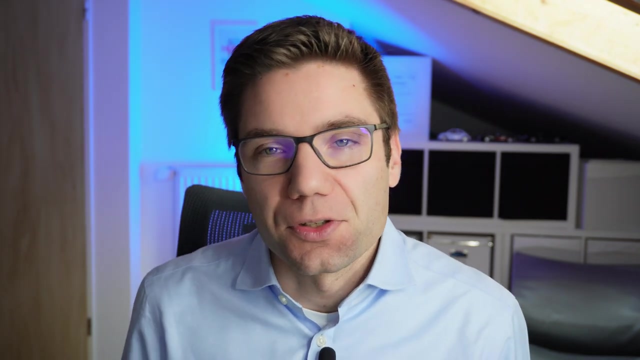 can do in this regard. if you want to take it even a step further. driving is easy compared to flying, so you could start building your first autonomous drone. there are not as many kits out there as you will find for cars, but you will find some instructions and 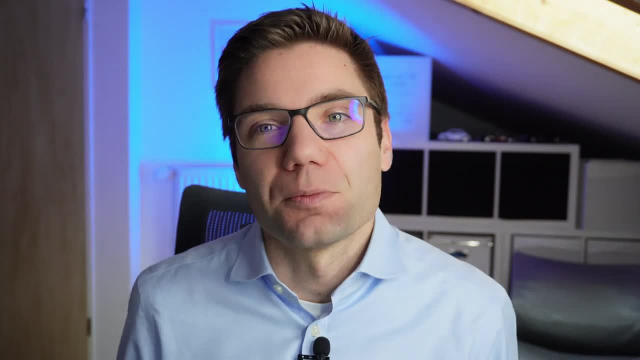 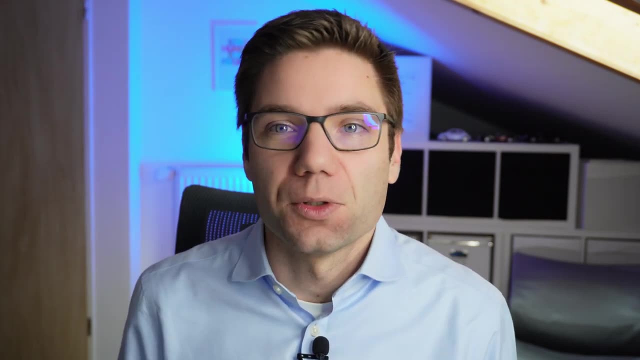 project ideas, especially on what hardware you need, and then you can start building your drone. one word of caution here: it's not allowed to fly those drones everywhere, so, depending on your country, there might be some regulations on where you are allowed to fly those, so please make sure. 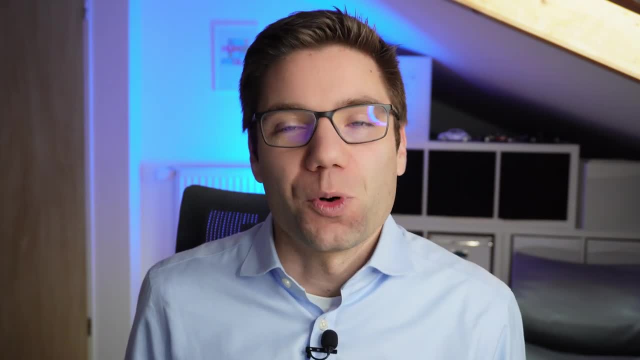 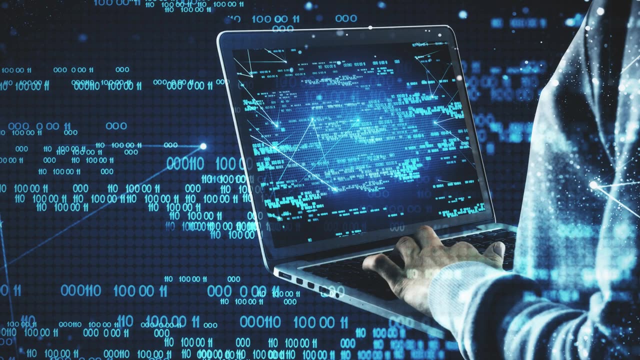 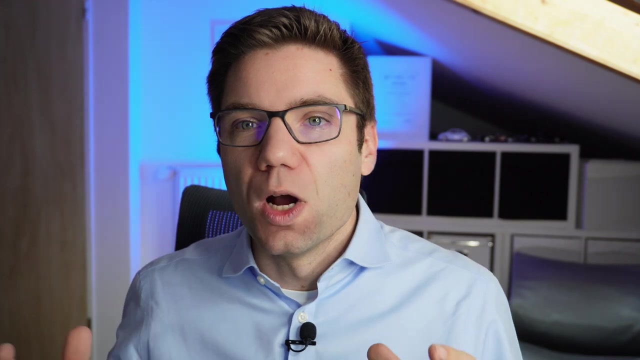 that you have understood those constraints before you get into trouble. And then, lastly, what you could build is a embedded operating system, and here you can also really take it from a beginner level scheduling system, where you just schedule tasks in certain time frames, to a much more complete. 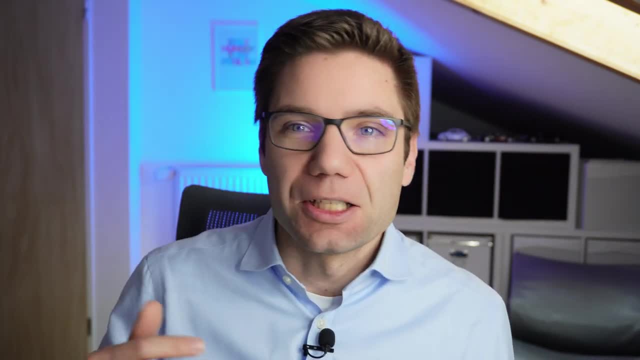 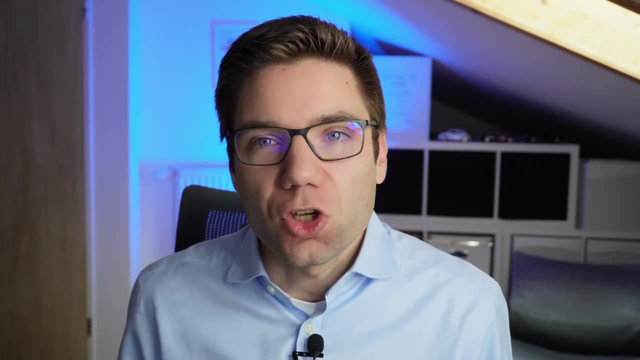 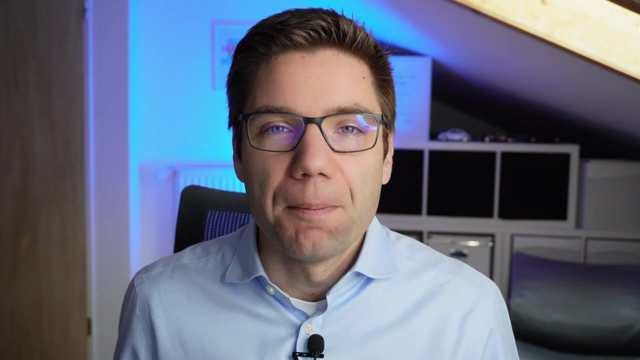 operating system with task handling, priority switching, memory management and much more things, and this is a great way not only to have more and more challenges and to iteratively build up the complexity level of your project, but also to understand the concepts of operating systems, because building your